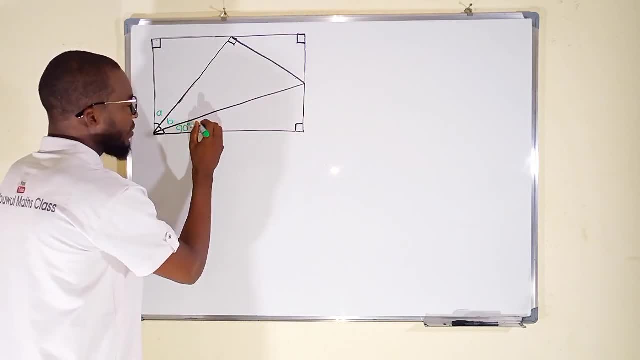 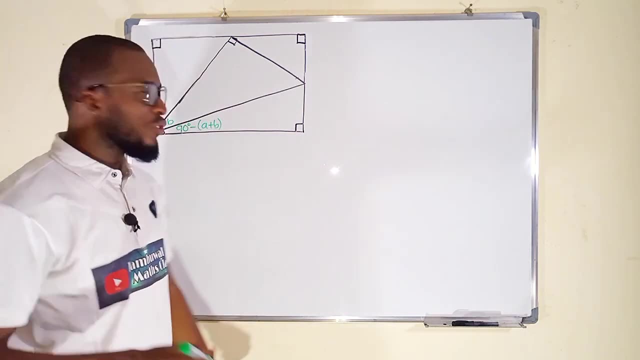 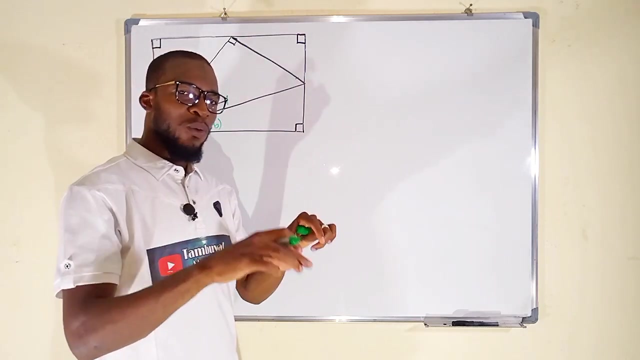 from 90 degrees. so this is 90 degrees minus the sum of A and B. let the hypotenuse of this right angle triangle be one unit. you know this is a rect angle. the interior angle: sum of two: 180, we have 90 here if you subtract that. 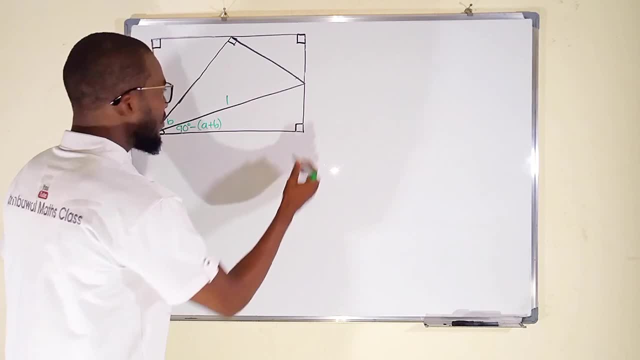 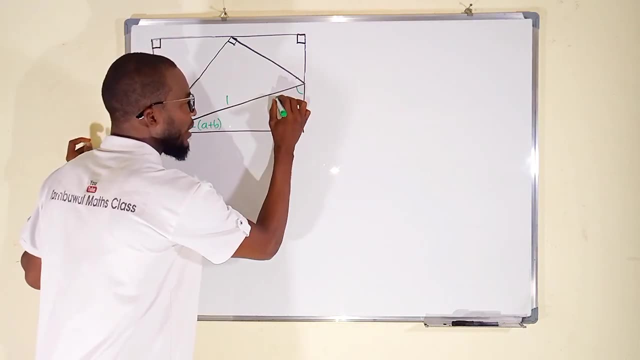 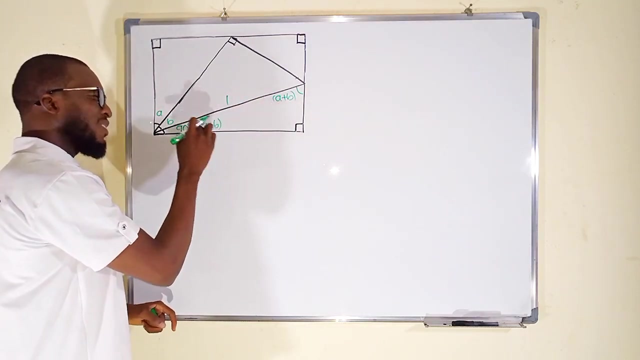 from 180, you get 90. this means that this angle plus this angle will give us 90. what does this implies? it implies that this angle will be a plus B, because a plus B plus negative, a plus B will give us 0, or we have 90 degrees plus 90. 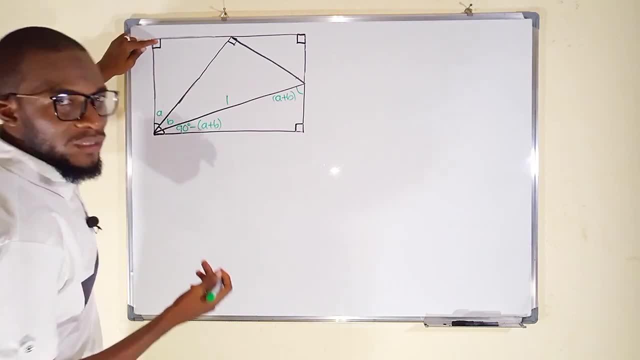 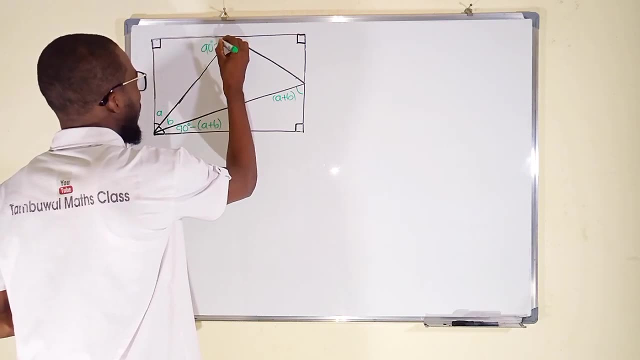 equals to 180. let's move on. this is already 90 degrees. this plus this will be equal to 90. so this will be 90 degrees minus a. this is another 90. you know I'm good on this right angle triangle. so this is 90 degrees minus a. this is another 90, you know. angle on the. 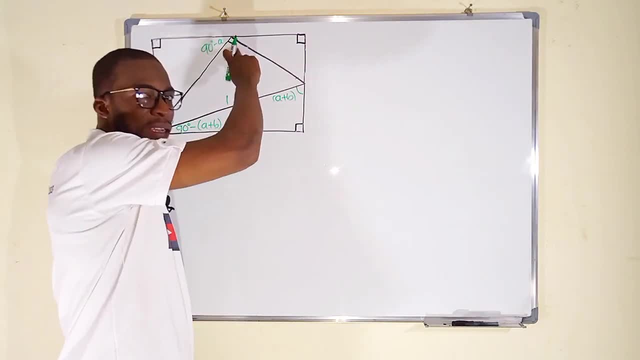 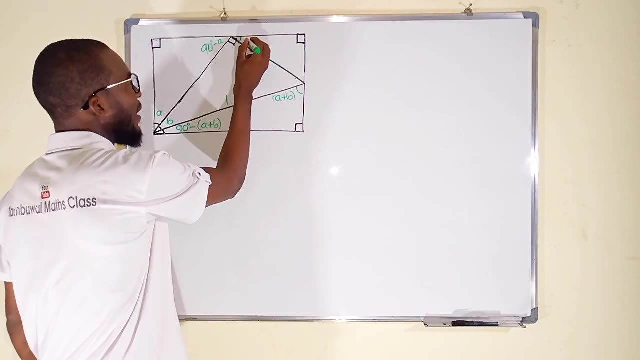 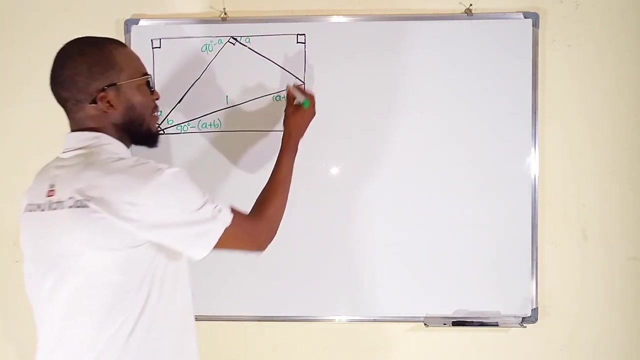 straight line is 180. we already have 90 here. what is left is 90. so this angle plus this angle will give us 90 degrees. therefore, this angle right here must be equal to a. we have another 90 here. therefore, this and this must be 90 as. 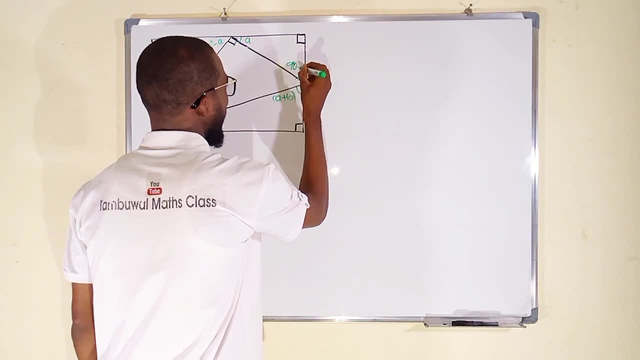 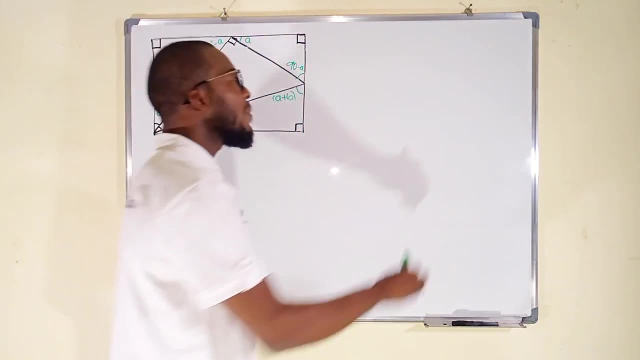 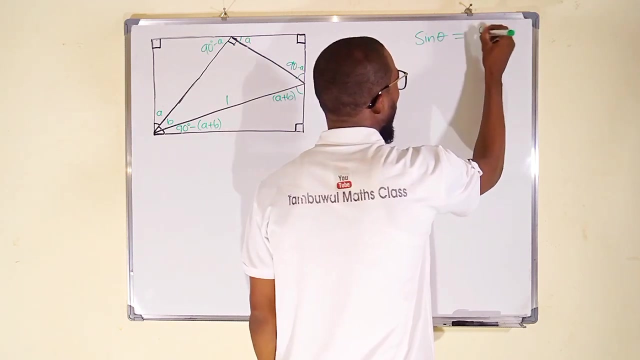 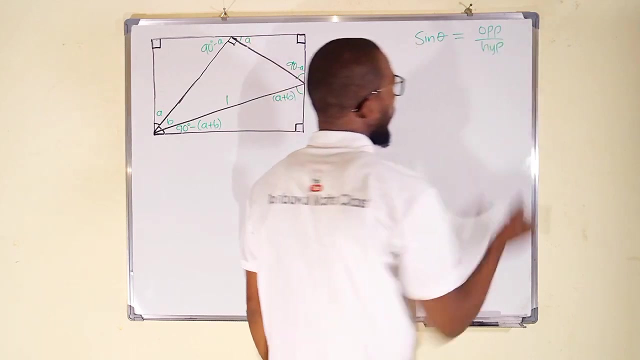 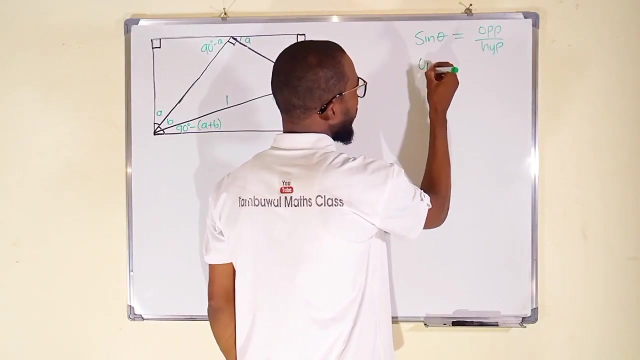 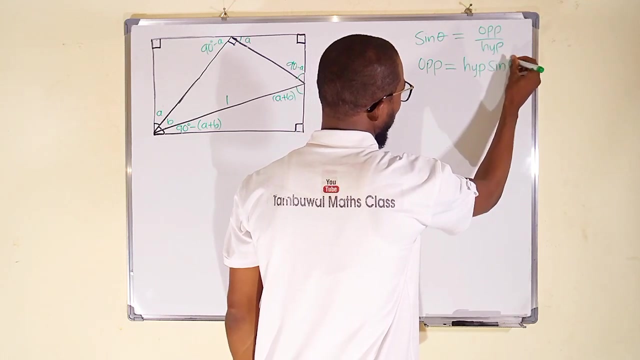 well, so we have 90 minus a. now let us go ahead and find the corresponding sides. but remember this: actually what happens is that it means that 2, the like for Zeit, equal to 90, three times the sign of an angle, is equal to opposite divide by hypotenuse. but if you are looking for the opposite, you can multiply the sin theta with the hypotenuse, so opposite will be equal to hypotenuse multiplied by sine of that angle. and for cos theta will be equal to 90 minus 1 plus 1他是 90, than Vanessaくせ um detail plus 90, which is 90, руб 100 meters. how much cost? 1 plus 90th or 1 is the sum of right and 1, same point of or. if you write the straight line or theOLBосả demand 2 smallest. when you multiply that with your нуженverses, you have a connection symbol. 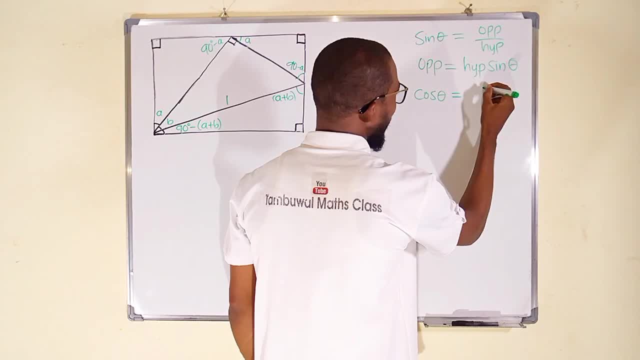 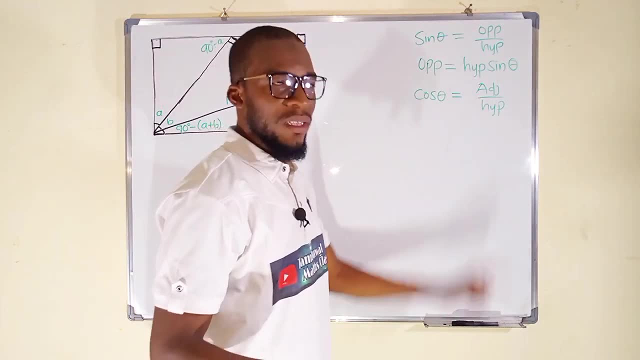 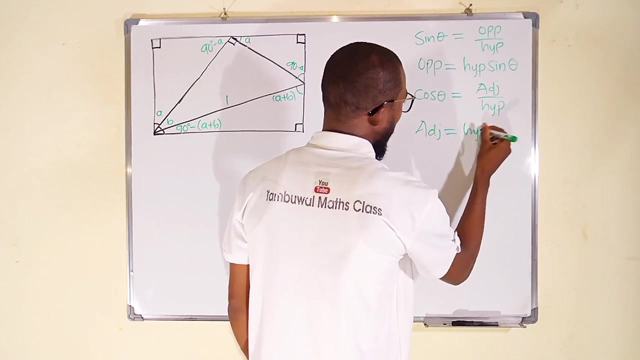 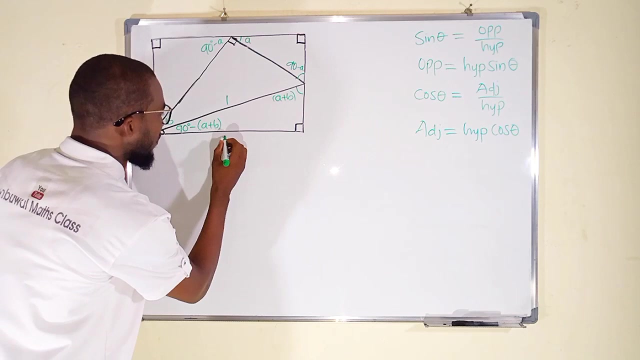 course of that angle. it can be obtained by taking adjacent divided by the hypotenuse and therefore, if you make adjacent the subject, you can obtain adjacent by multiplying hypotenuse by course of that angle. so let's continue. let's start with this side. this side is directly opposite to the side and 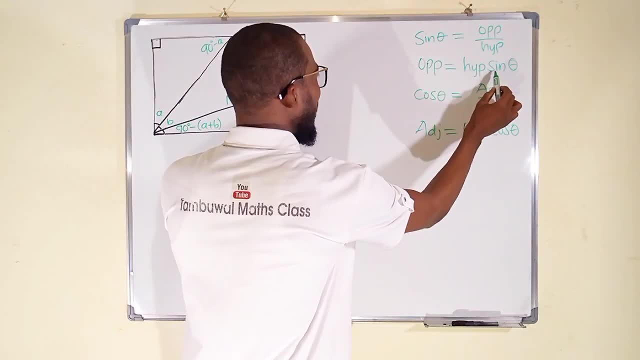 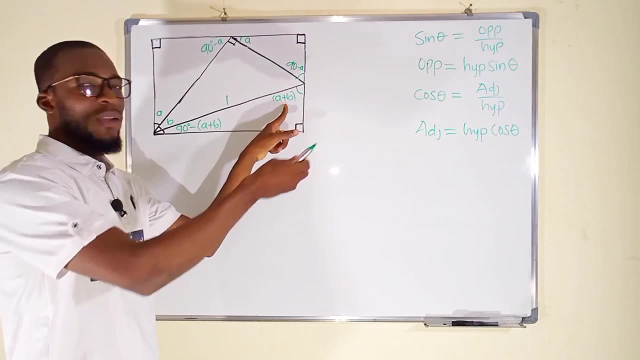 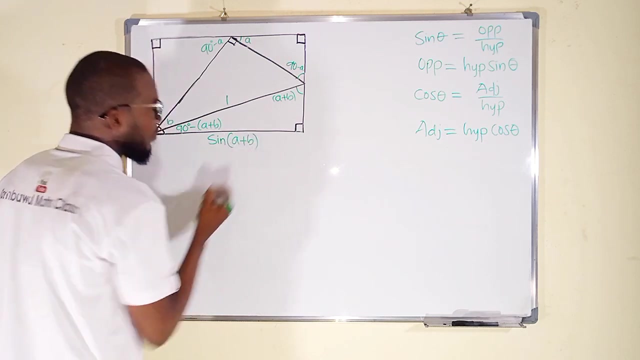 opposite can be obtained by multiplying the hypotenuse and the sign of that angle. the hypotenuse is 1 multiplied by sine of that angle. 1 times that sine will still be the sine of that angle. so this is sine of a plus B. let us move to. 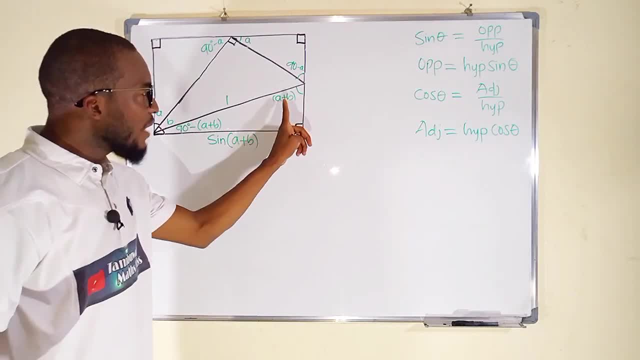 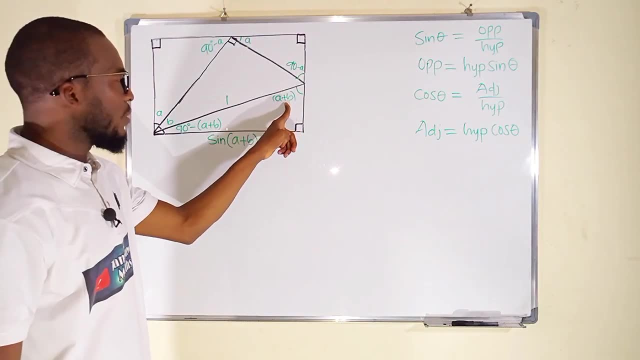 this direction. this side is actually the opposite of the angle. so this is sine of a plus b. so this is sine of a plus b adjacent to this angle. and adjacent can be obtained by multiplying the hypotenuse with the course of that angle. hypotenuse is already 1 multiplied by. 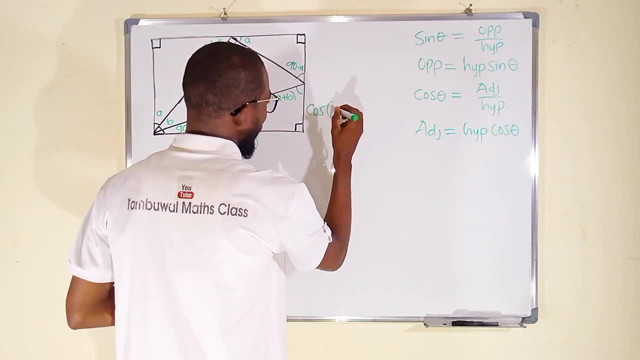 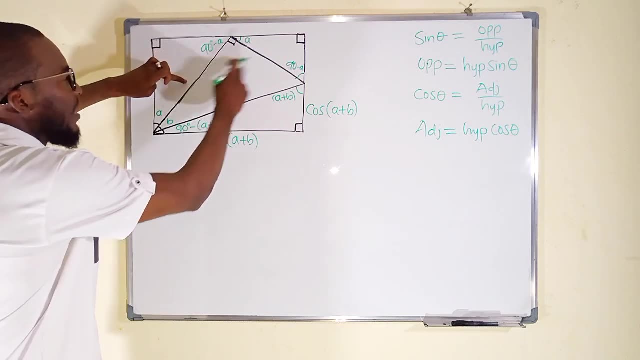 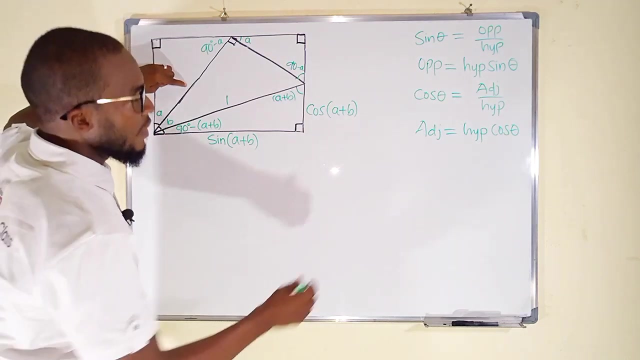 course of that angle, it will still be because of that angle. okay, let us find this side and this side. you can see that this length side is adjacent to angle B. adjacent is hypotenuse and the hypotenuse is 1 multiplied by cos of that angle, the hypotenuse is 1. 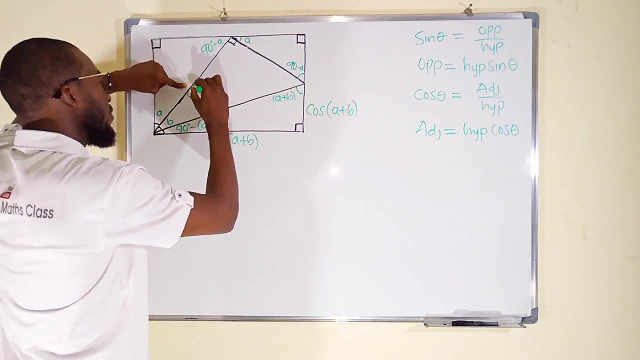 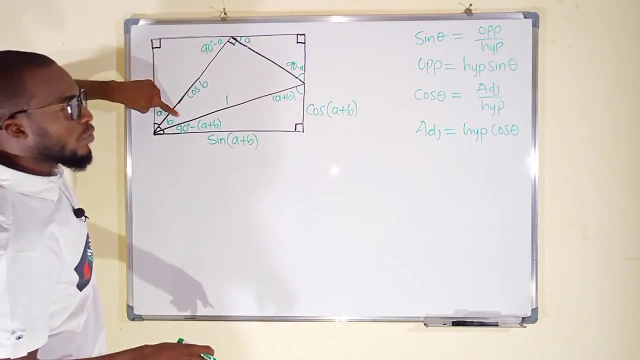 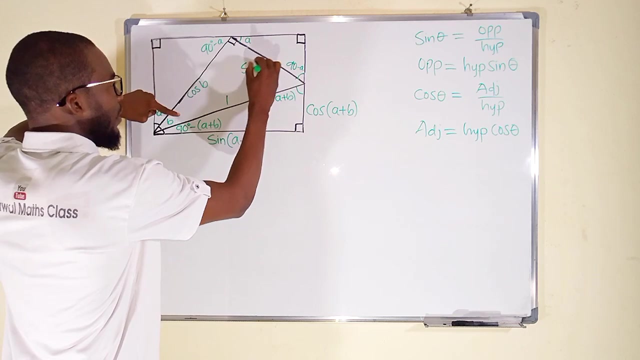 multiplied by cos of that angle. so this is going to be cos cos B. this one is opposite to this angle. opposite is hypotenuse multiplied by sine of that angle. so 1 multiplied by sine of B. we still have sine sine B here. now let us 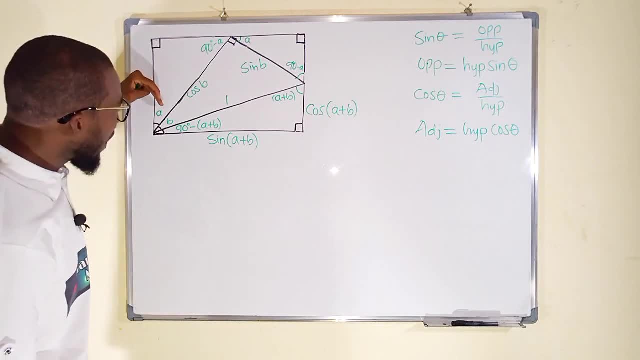 find this side length. this side length is adjacent to this angle a, and adjacent can be obtained by multiplying the hypotenuse and cos of that angle. cos of that angle, you can see, is cos A multiplied by cos B. so this becomes cos A, then cos cos B. what about this side? this side is directly opposite. 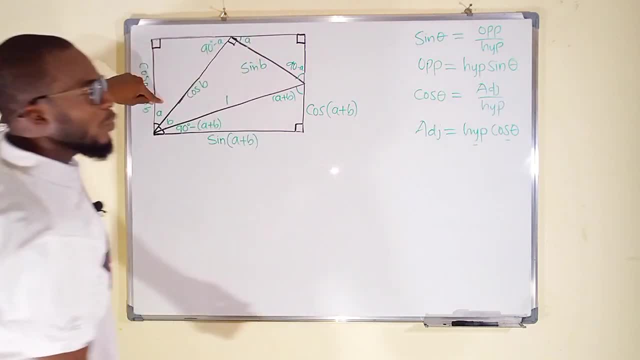 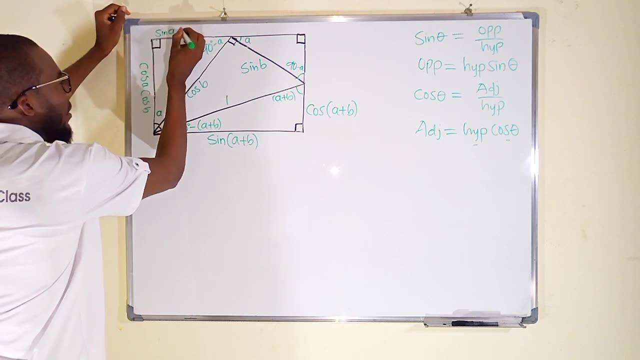 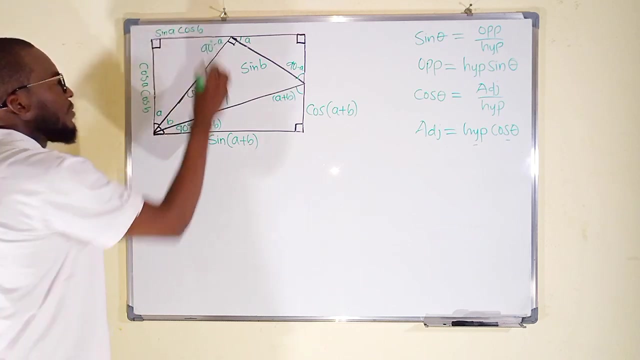 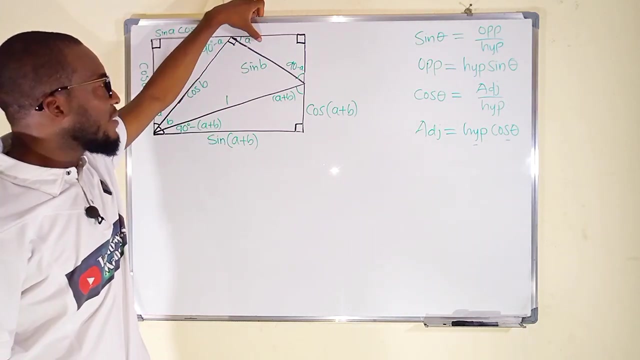 to angle a, opposite, you can see it's hypotenuse multiplied by sine of that angle. this is of that angle. so, sine of that angle, sine of a, they are multiplied by the hypotenuse, which is cos, cos b. let's move on. let's find this side length. this side length is directly adjacent to angle a. 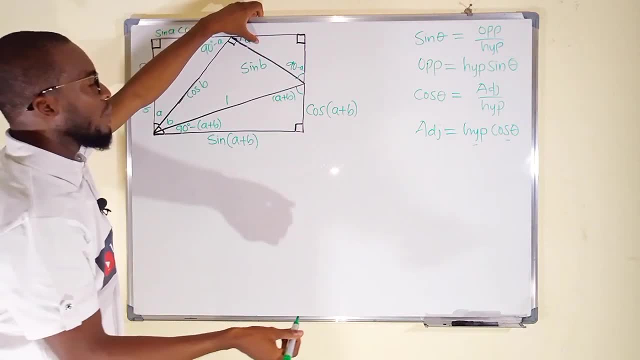 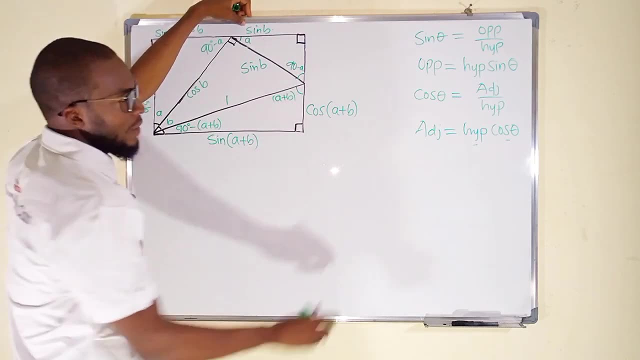 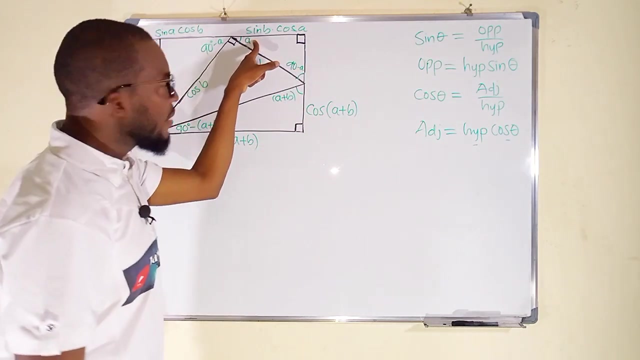 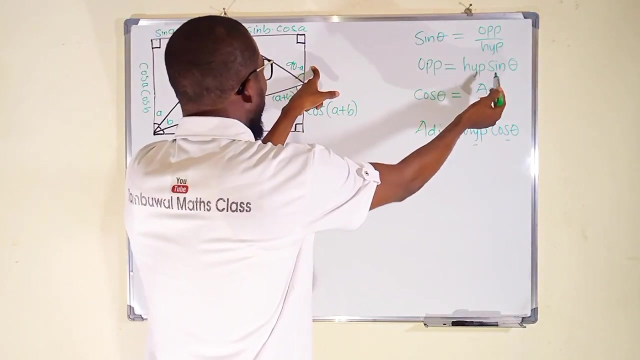 adjacent, is hypotenuse multiplied by cos of that angle. so this is the hypotenuse sine b multiplied by cos of that angle, cos a, so we have cos a here. and last but not the least, you can see, we have this side length which is directly opposite to angle a. opposite is hypotenuse multiplied by sine of that angle. 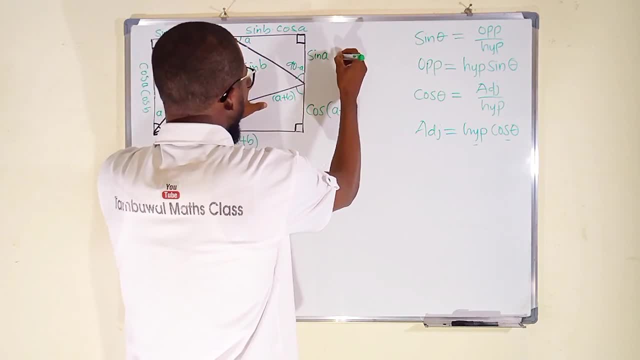 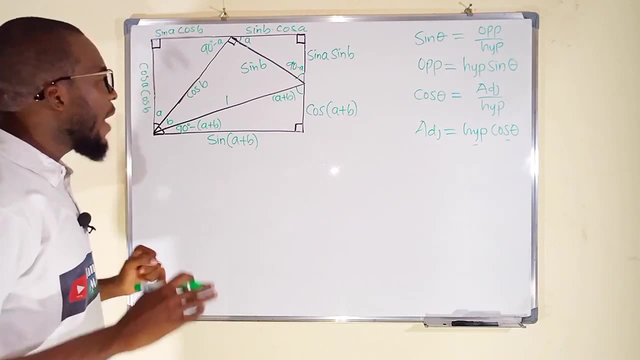 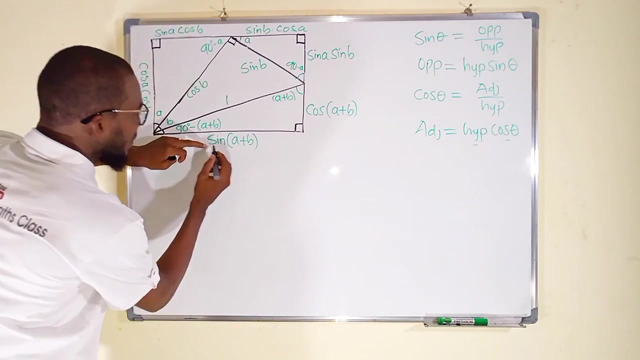 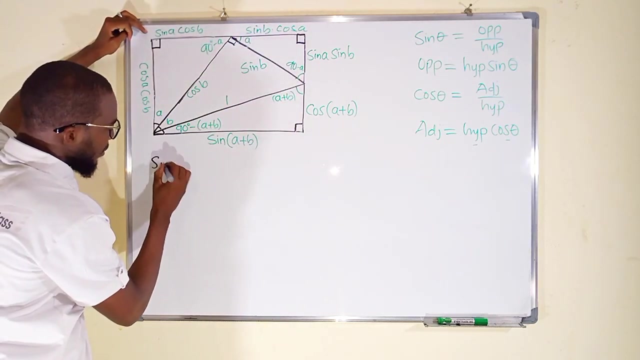 so we have sine of that angle, a, multiplied by the hypotenuse which is sine b. now we have obtained this side length of a plus b plus sine of that angle, and of course sine of that angle is 90 and equal to sine of that angle, equalsore and equation we have right here. 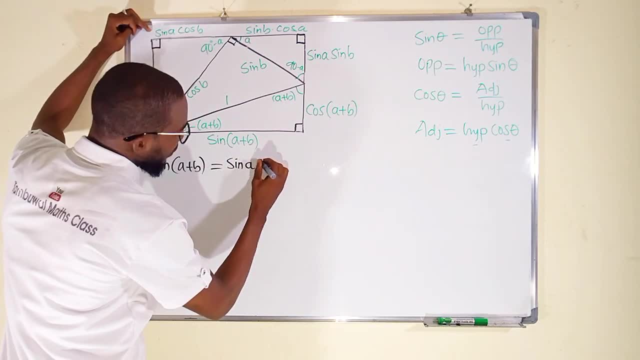 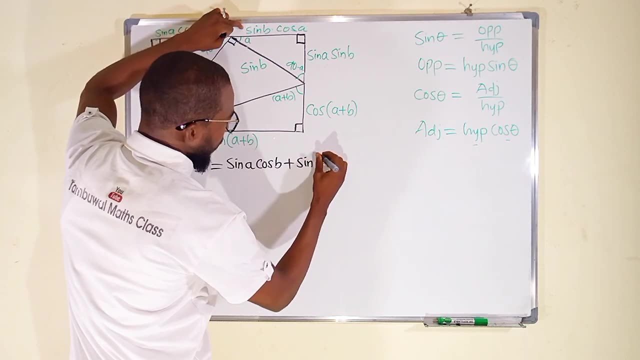 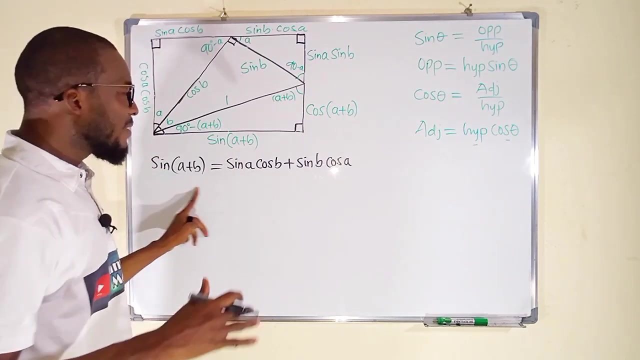 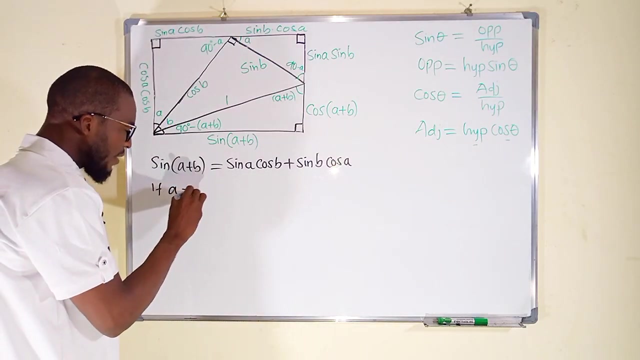 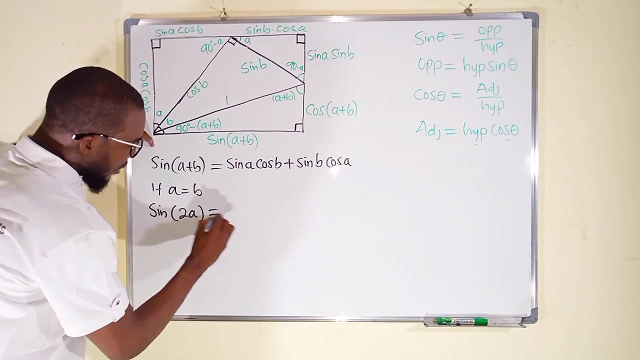 this is the relationship between sine of the angle and the fine from the gyrate need to be a sine B, cos cos a, so to obtain double angle. this is the right formula to use. but what if a is equal to B? if a is equal to B, this becomes sine 2: a equals. 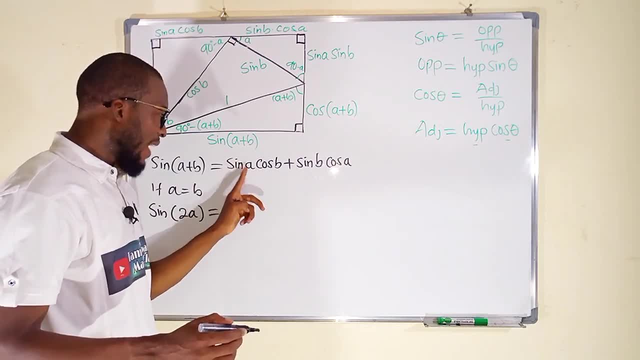 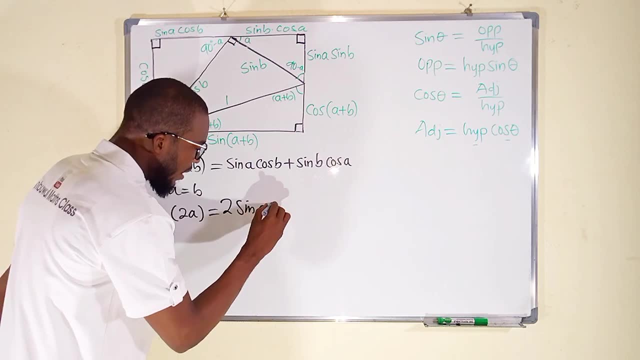 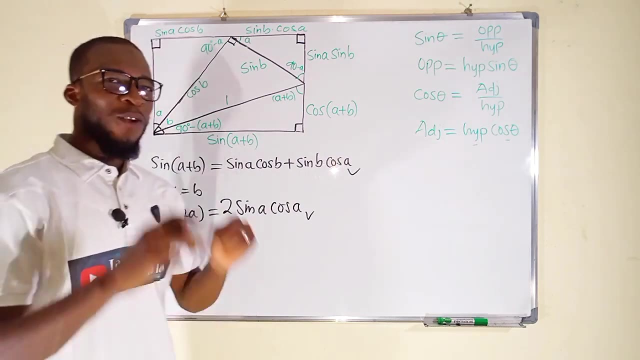 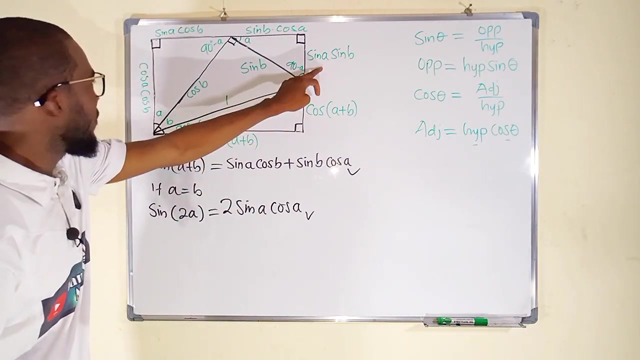 if a is equal to B, we have sine a cos a, sine a cos a, making 2, sine a cos cos a. can see one here. you can see the other one here. these two formulas are very essential. now let us derive other ones. this other sides are equal, so we can see that this plus this is equal to this. so we have. 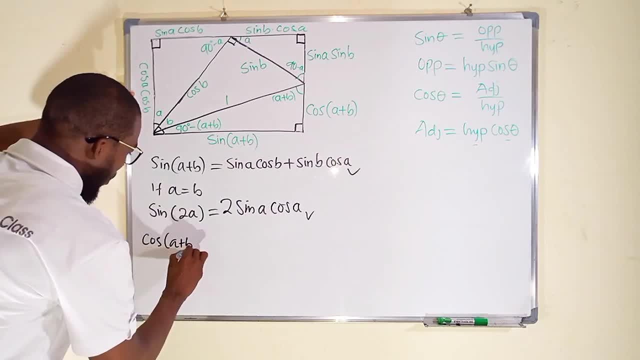 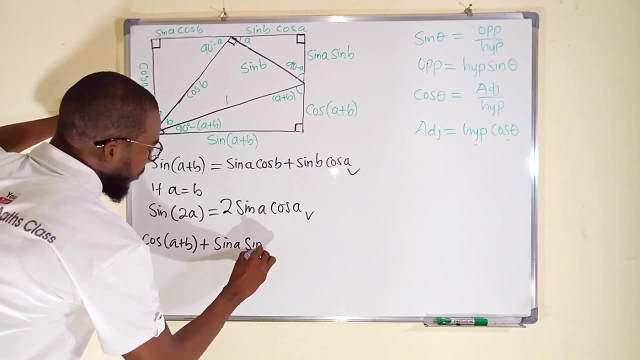 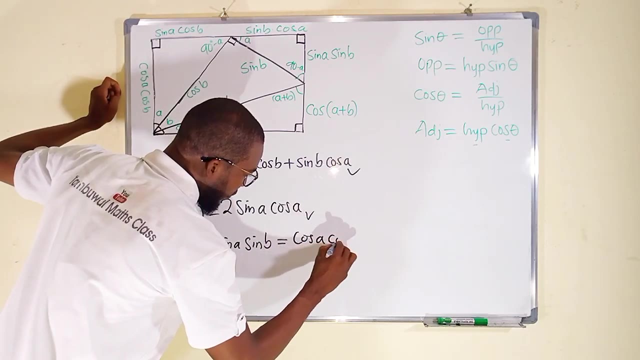 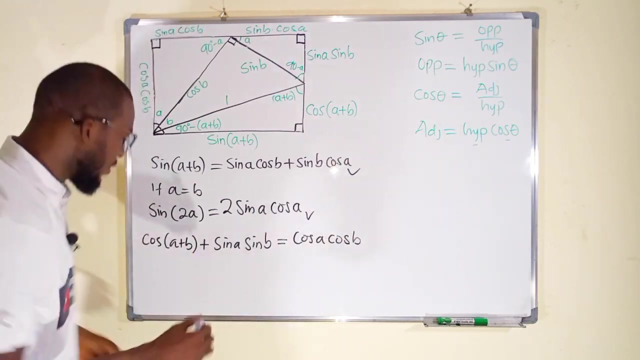 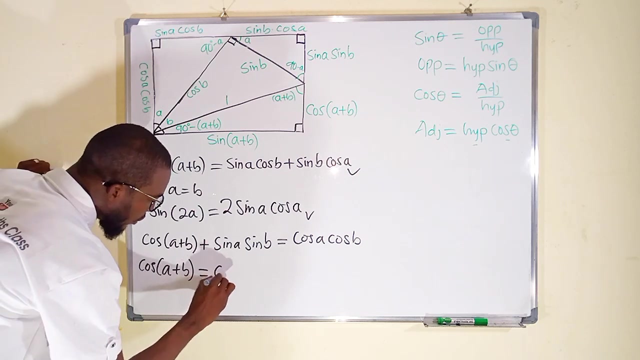 cos A plus X, cos A plus X, B plus sine sine a, sine B. this is equal to cos a cos B. cos a cos cos B. since we are interested in knowing the double angle, you can take this one to the right. so we have cos a plus B. equals what we have there to the right: cos a cos B. 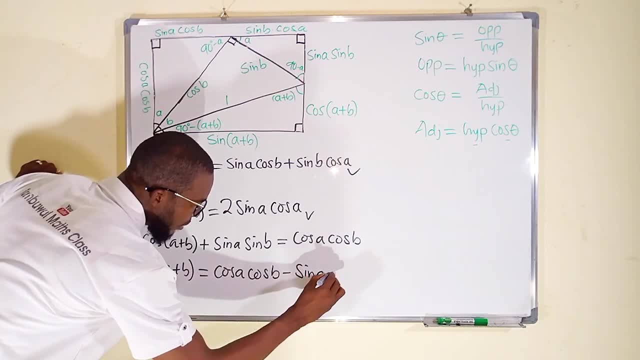 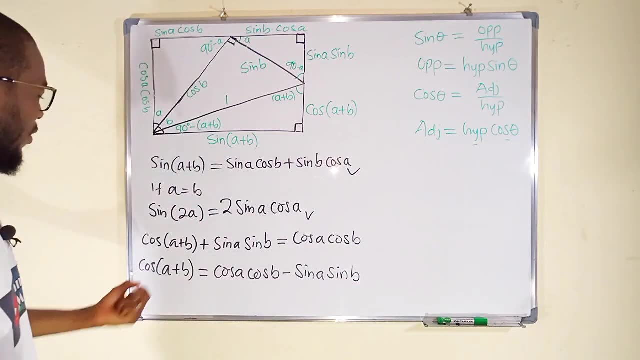 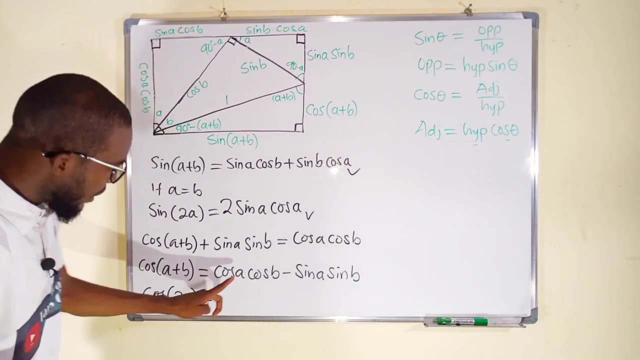 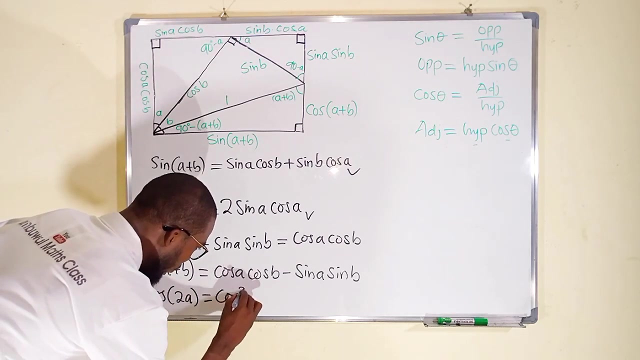 minus sine a, sine sine B. and if a is equal to B, we can obtain another double angle here. cos of 2a will be equal to. if a is equal to B, we have cos a multiplied by cos a, cos squared a, so we have cos squared a here. 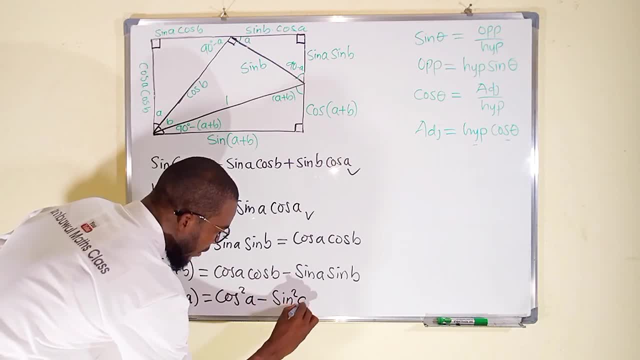 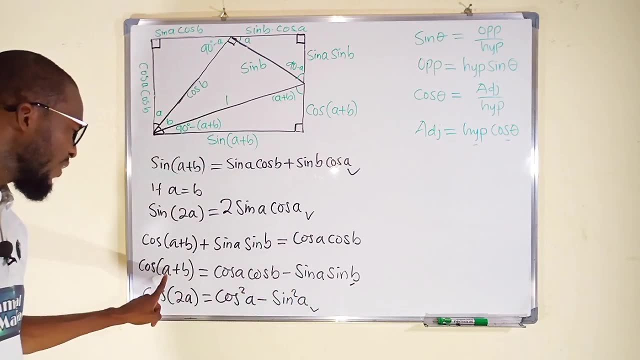 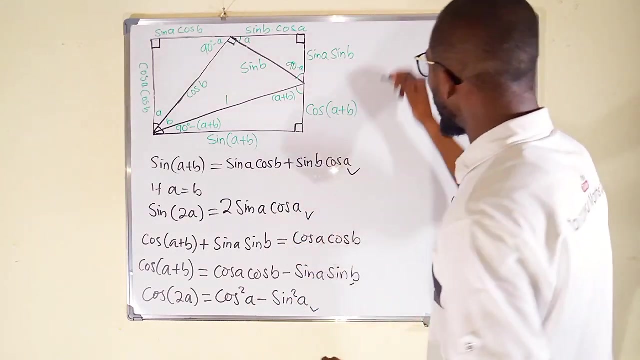 minus sine squared a. you can see another important formula here. we have two of them. in case, if the angles are different, you use this formula, but if the angles are the same, you use this other formula. we can still find some from fatigue rule. it says that hypotenuse squared, which is 1 squared, is: 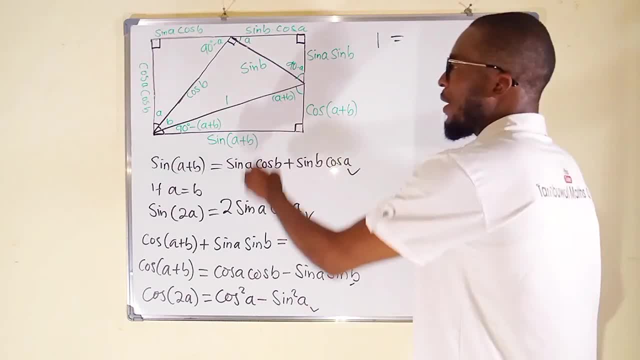 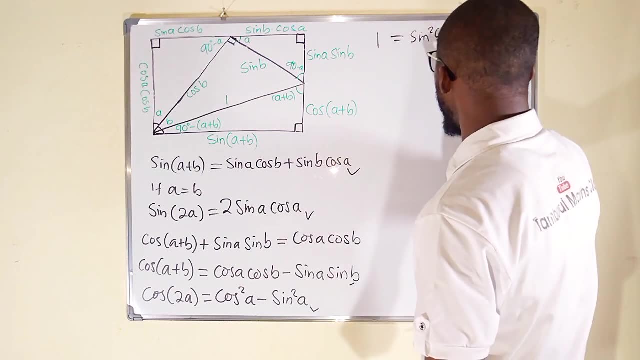 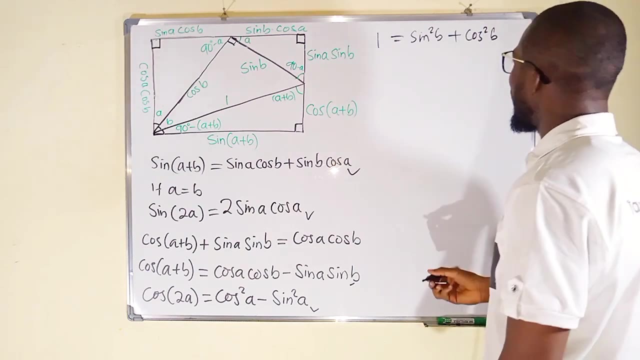 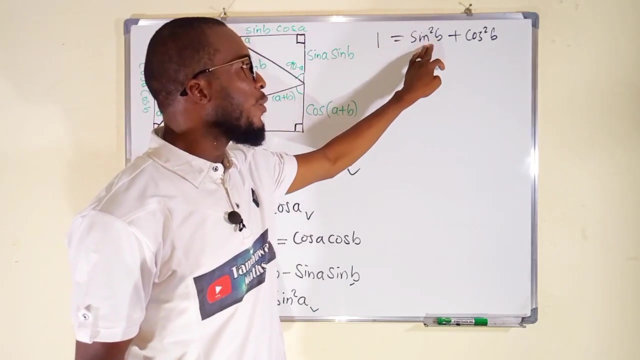 the same thing as 1 is equal to opposite squared, which we have here as sine B squared, sine squared B, plus the adjacent squared, which is cos squared B. look at another identity which is very important: if you have cos squared and angle plus sine squared of the same angle, the result will always be equal. 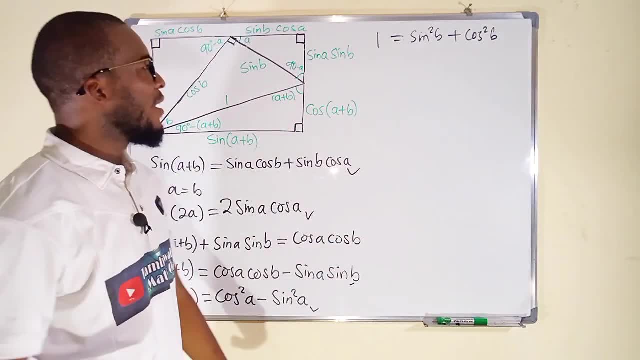 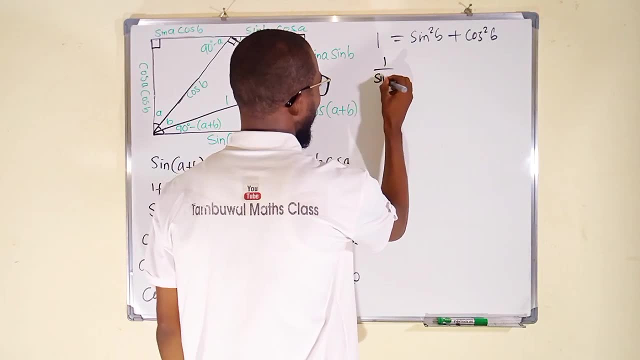 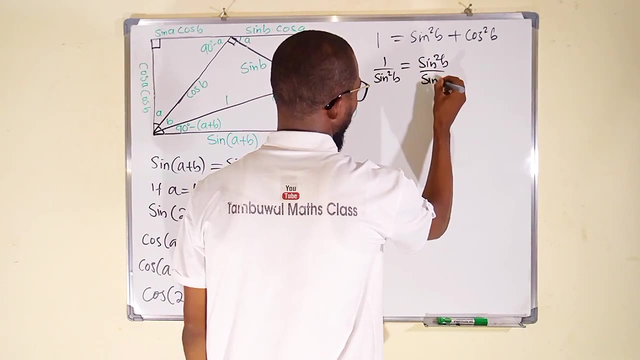 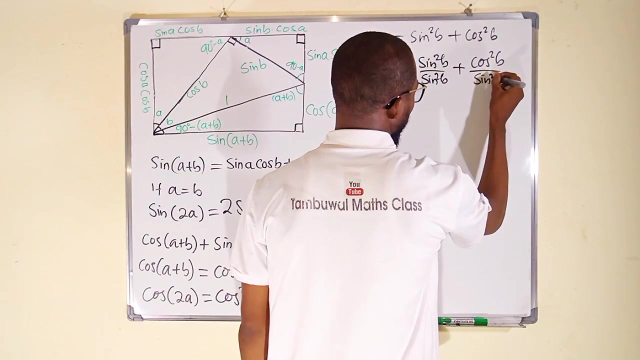 to 1 and from here we can derive other identities. let us divide each time here by sine squared B. so we have 1 divided by sine. squared B equal to sine squared B divided by sine squared V plus cos squared B divided by sine squared B. squared b, reciprocal of sine, is cosecant. because this is squared, we have cosecant squared. 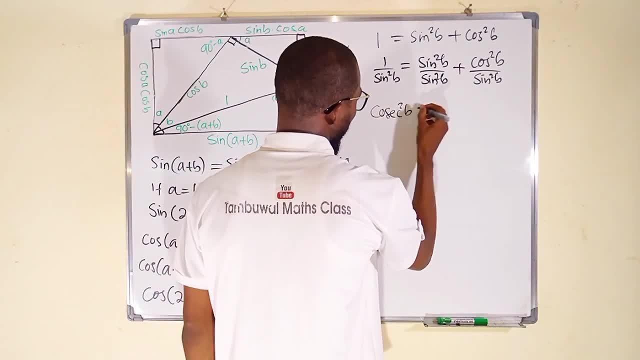 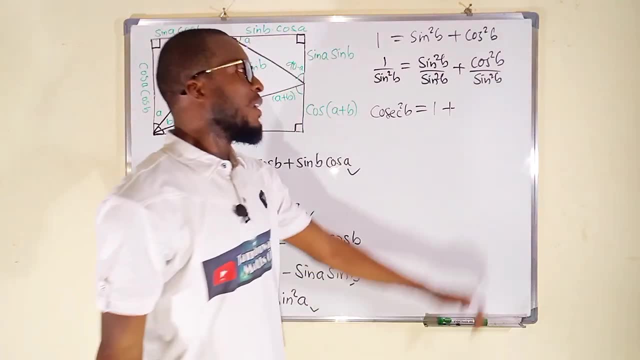 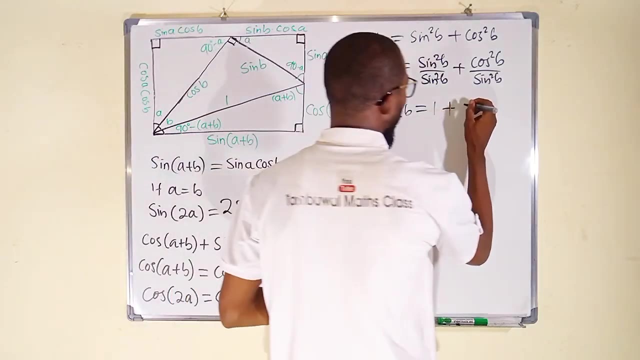 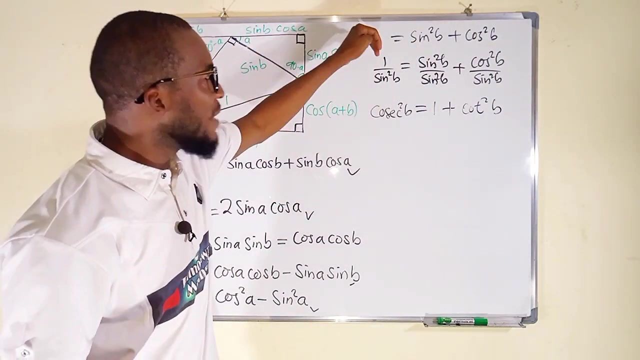 cosec squared b equal to sine squared b divided by sine. squared b is one plus. remember: sine over cos is tan, but cos over sine is cotangent, but this time around we have code squared b. look at another identity driving from the initial one. if we like, we can divide. 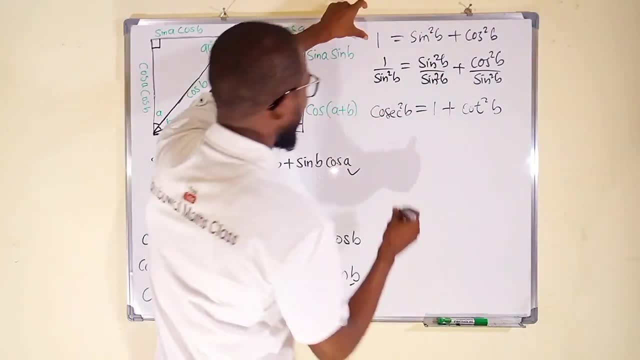 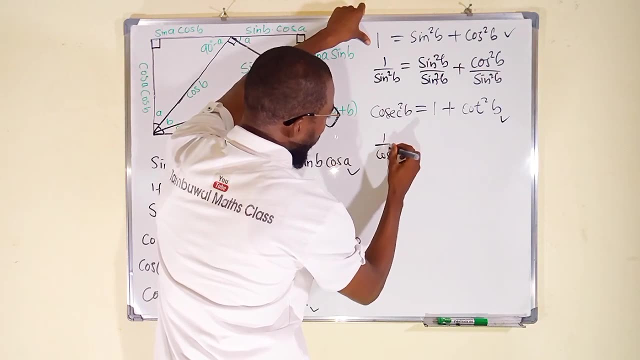 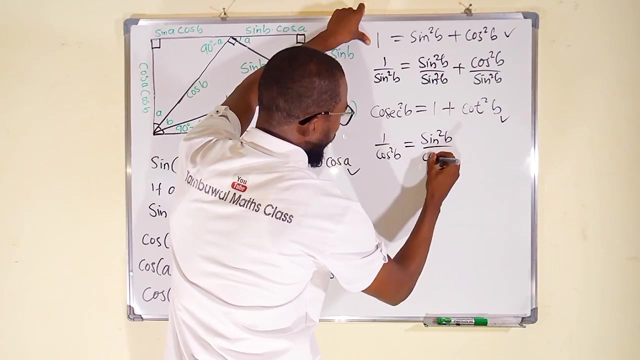 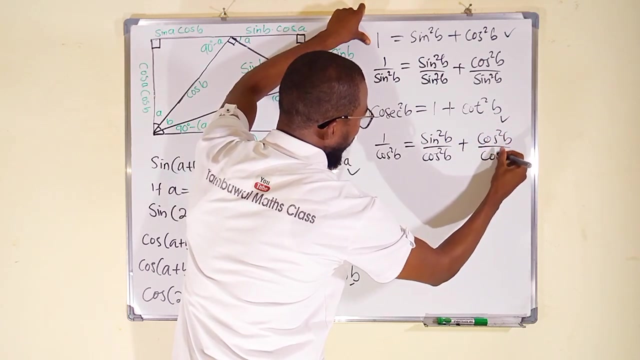 each time by cos squared b to obtain another identity. let us do that we have. this is important. this is important if we have: 1 divided by cos squared b, equal to sine squared b divided by cos squared b plus cos squared b. squared b divided by cose squared b, reciprocal, of course, is sec. so we have 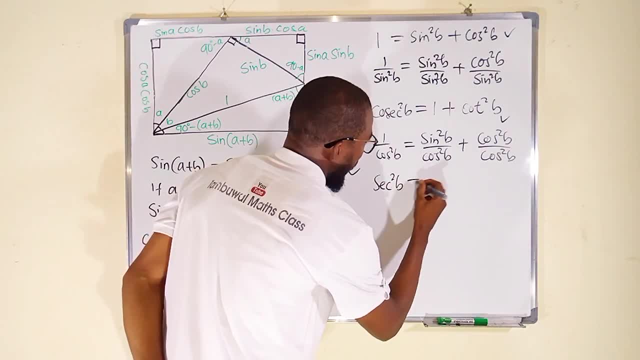 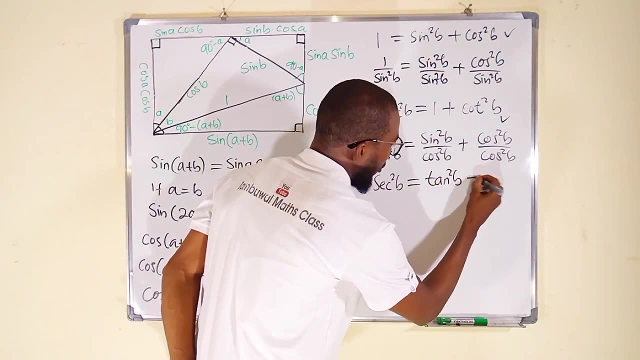 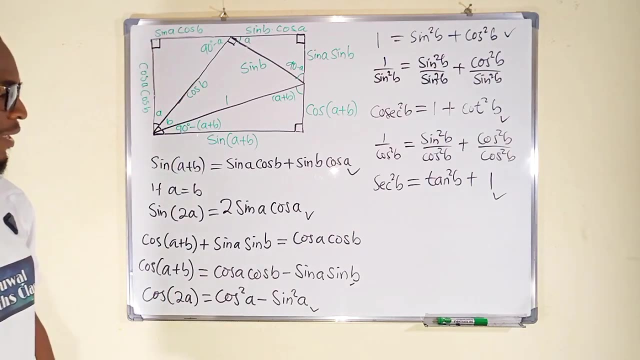 second: squared b equals sine over. cos is tan, but this is squared. we have tan squared b plus cos. divided by cos is 1. look at another important identity. we have driving 1, 2, Three, four, five, six, seven. Let me see I can drive other ones from this one. Look at it here. 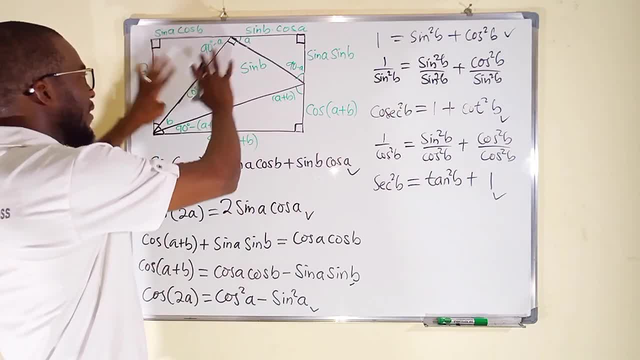 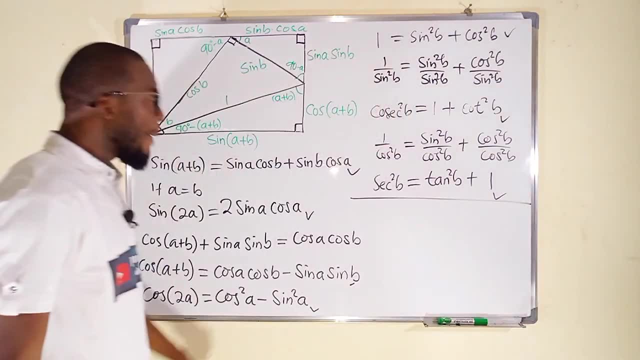 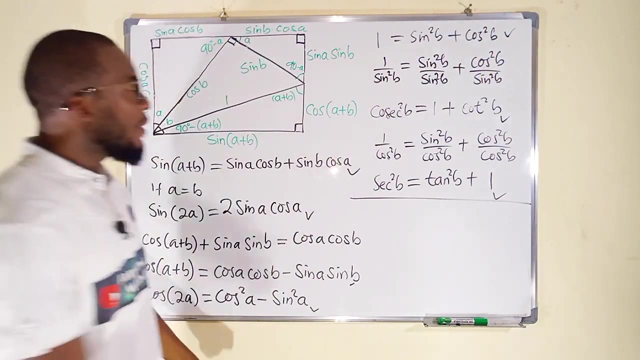 I can drive other ones from this one, So let me take this diagram down because we don't need it anymore. But let me use this face. We have seen that sine squared B plus cos squared B is equal to 1. this implies that sine squared B is: 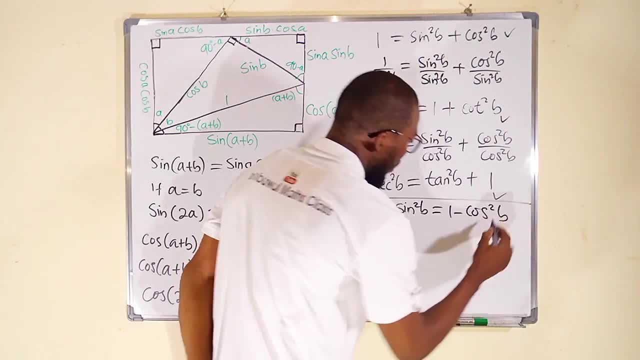 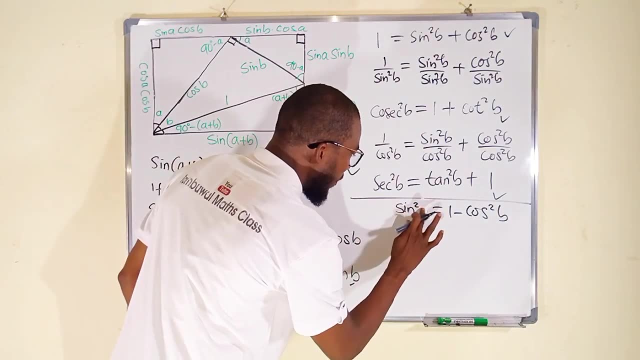 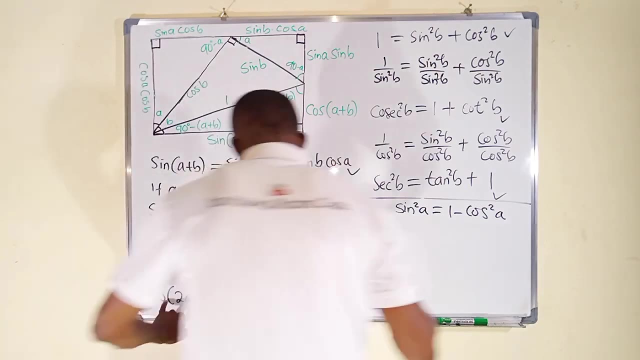 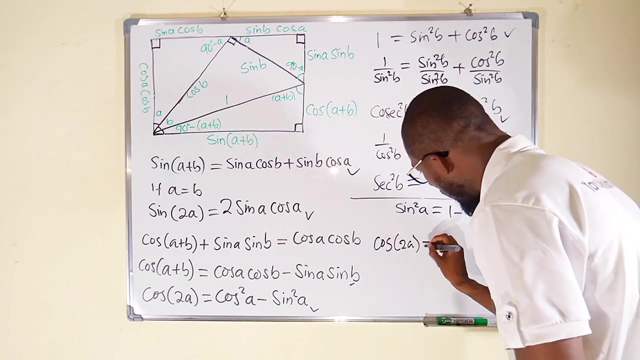 equal to 1 minus cos Squared B. Let us substitute this information right here, Where we have a here instead of B, So I can write this one as a. This is a as well. Let me substitute it here. This becomes Cos 2, a equals. we have: